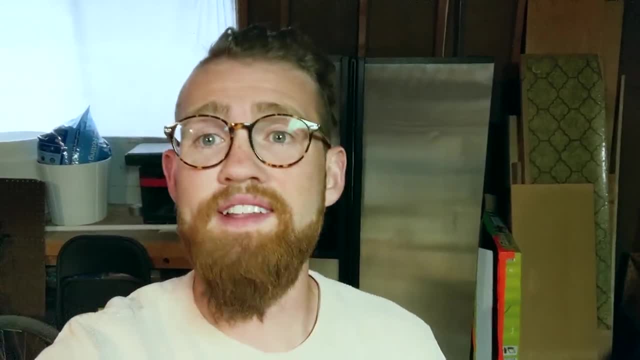 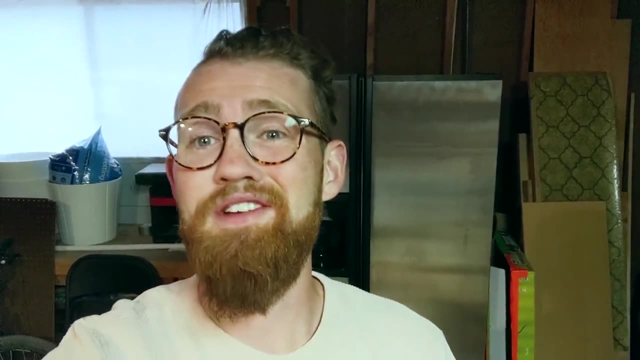 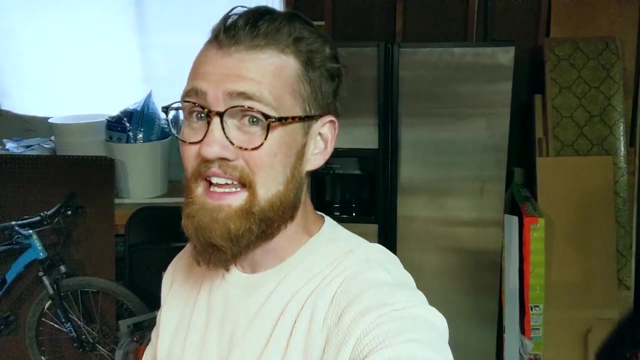 time. stay tuned, because I'm going to be talking about all the different cuts, how much meat I got, what we saved and what our plans are with the rest of our lamb. So stay tuned. I mentioned it at the beginning. I'm going to just say it again. just to say it. Don't judge me. 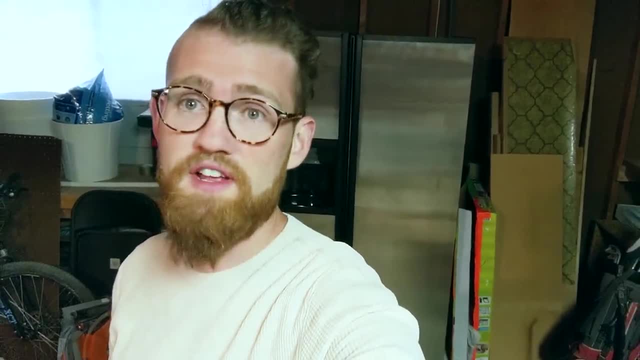 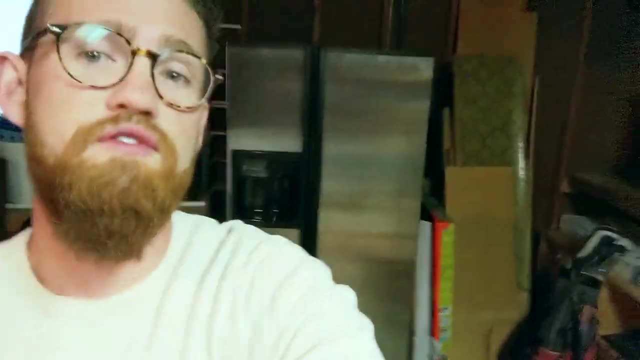 for my messy garage. It is what it is. We moved in almost a year ago. We don't even park cars here, You know why? Because the doors don't work, So it's kind of just like a storage unit for us. Okay, so here's what happened. I had two. 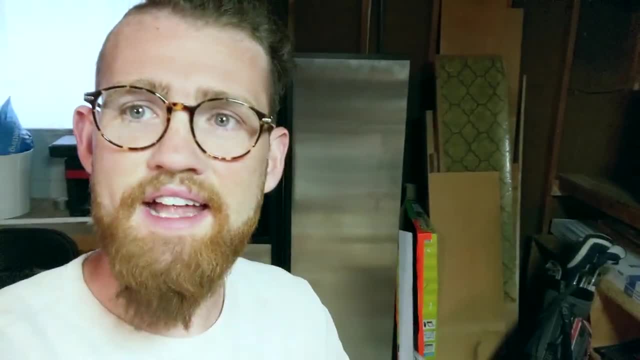 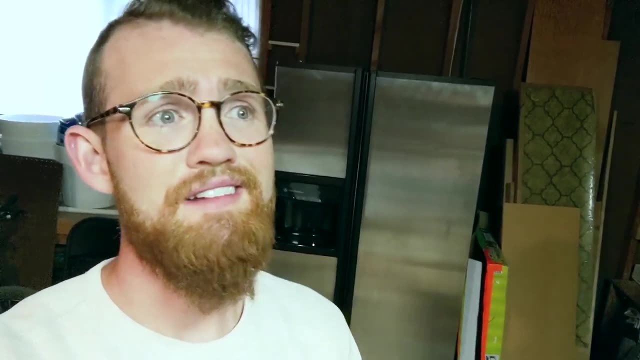 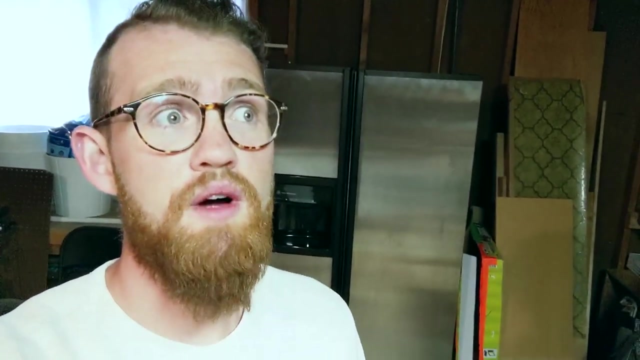 lambs, these two rams, and they were both almost six months. I would have liked to have waited a little bit longer But, looking back, I'm really glad that we processed when we did, Because my first two rams I got- one of them was 54 pounds, One of them was 54 pounds And I got one of them. 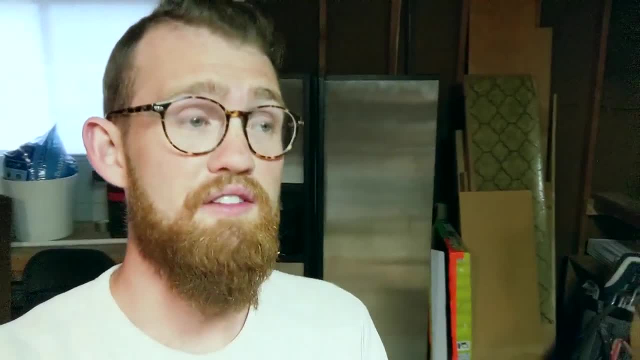 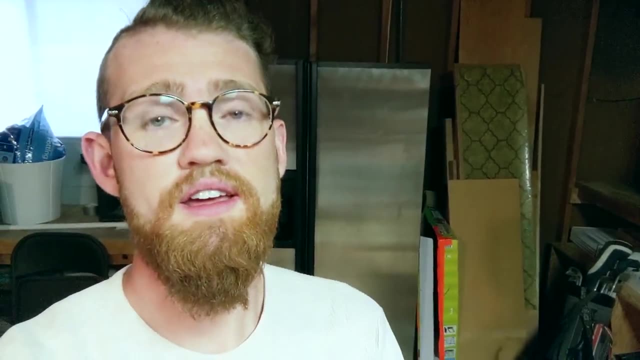 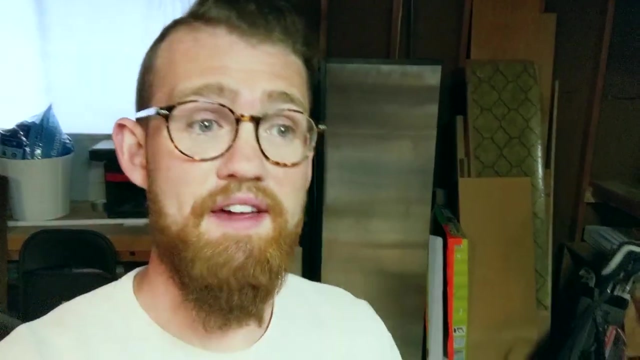 was 58 pounds And that is hanging weight, Really good weight for these rams. I'm really really pleased at a five and a half month ram to get that much weight. So let me talk about what the 58 pound ram actually gave us. My 54 pound I gave to my neighbor, so I don't have any of his. 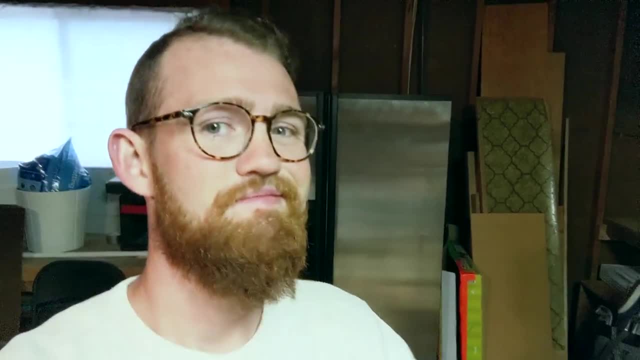 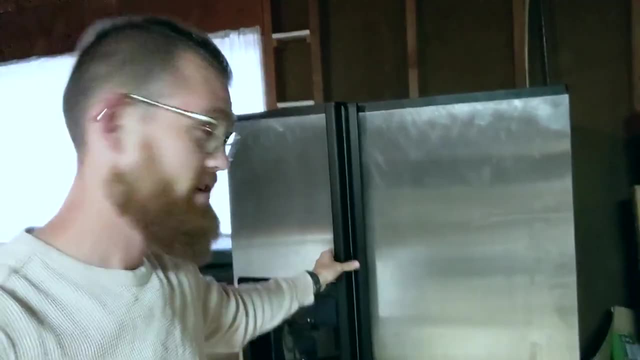 stuff lying around, But the 58 pounder totally got him in this freezer, So let's check it out Also. thank you, mom and dad, for giving me your old freezer. Congratulations on your new fridge. Really happy for you guys. All right, here we go. 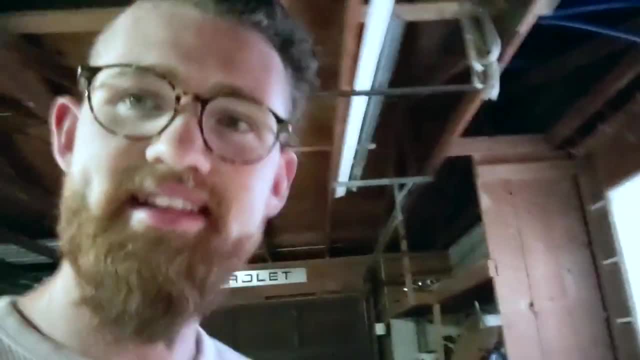 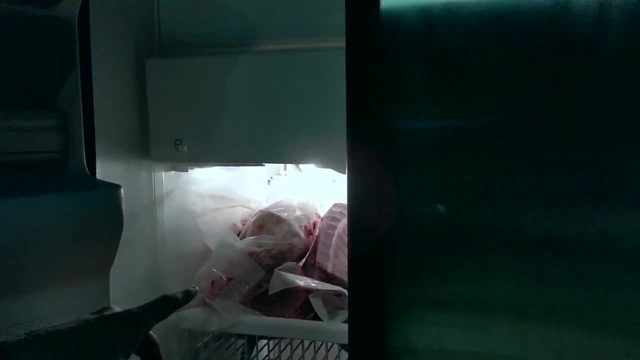 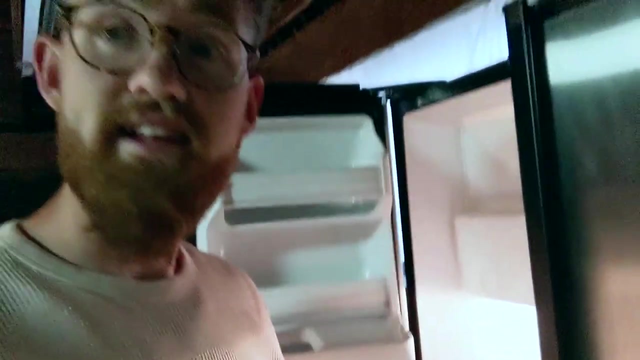 Got this awesome bike wagon that's keeping me from opening the door all the way, But that's cool. So up top I've got kind of like the stakes and more fancier things. Why don't I just get them out? I'll just show you what it all looks like. So, like I said I got, it was 58 pounds hanging. 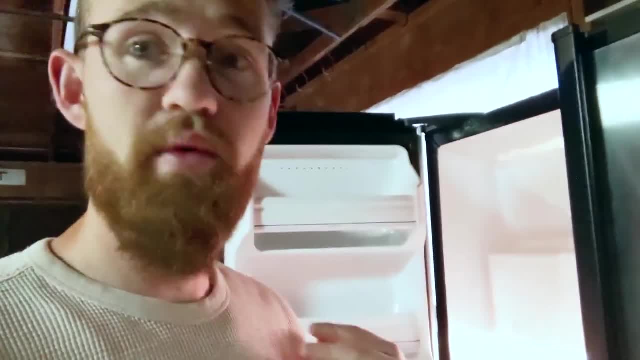 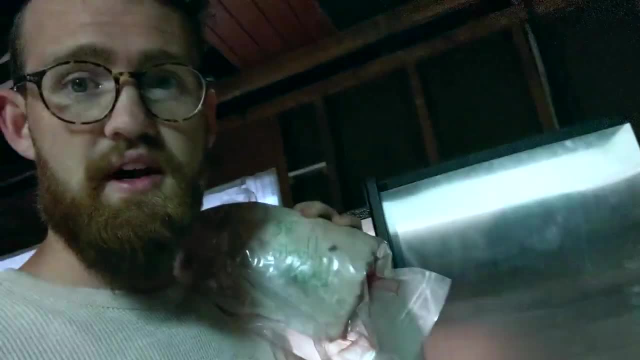 weight And we pretty much take everything out of the fridge, So I've got a little bit of a hanging weight. We don't want anything going to waste. So let's see what we got First cut of the day. That is the shoulder that we got right here. This is the skull And I will tell you what we're. 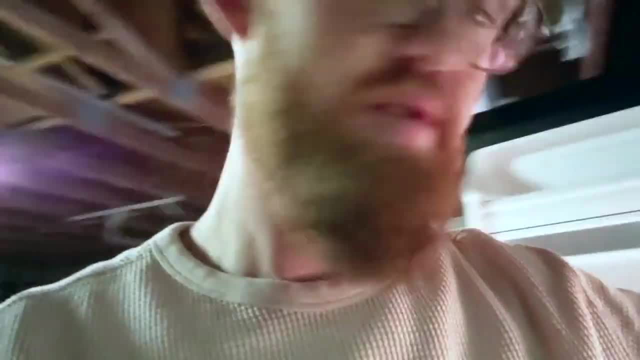 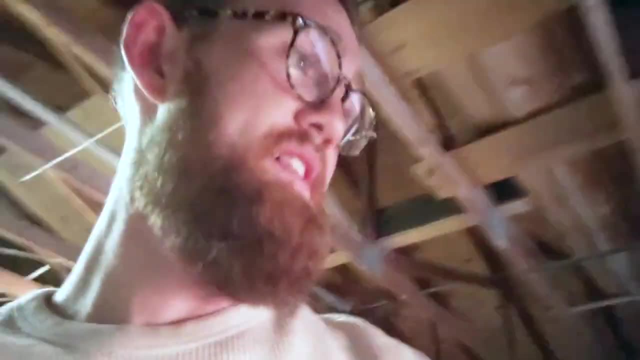 doing with that later. It's not what you think. If you think it's soup, you're incorrect. It's another shoulder, Another shoulder, roast right here. I guess that makes sense. There's four shoulders And another shoulder. Okay, bam, Got the shoulders. Oh my gosh, I've got a lot of. 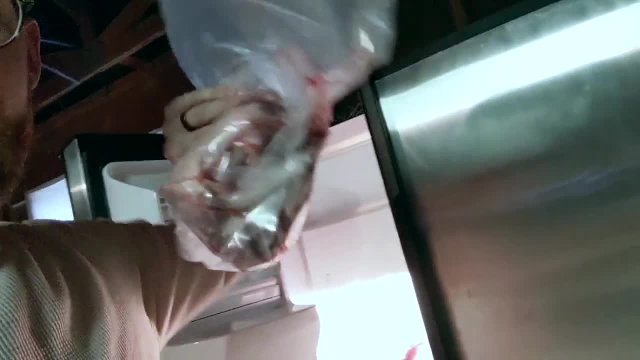 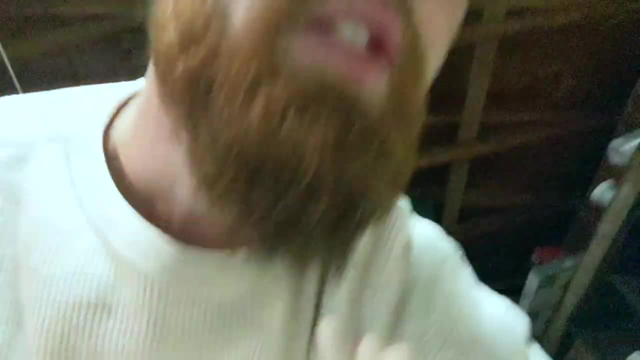 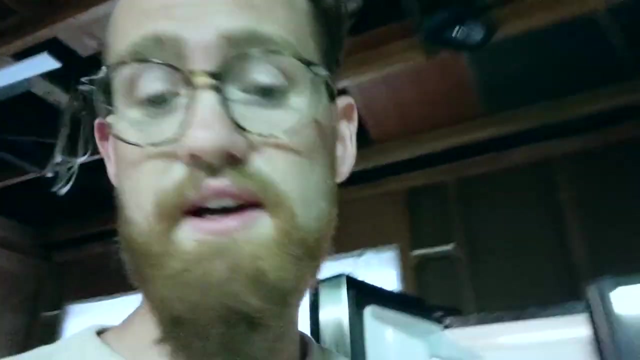 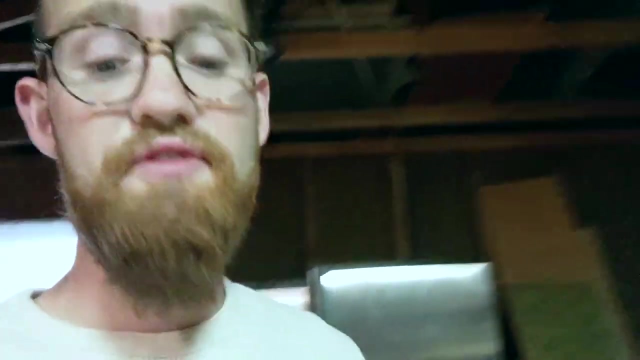 gosh, right there, That's shank, The lamb shank. Oh my gosh, So excited about that. My favorite part: the steaks. All about those leg steaks. So when we picked up these guys on Saturday they were not frozen, which was very cool. Brought this on Friday And then we picked up on. 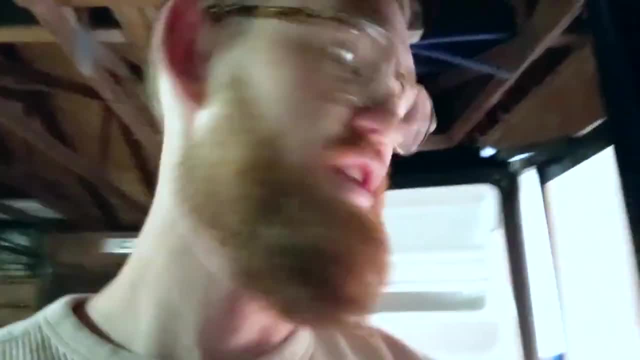 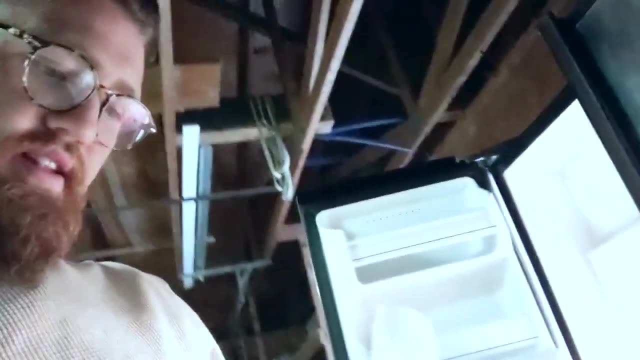 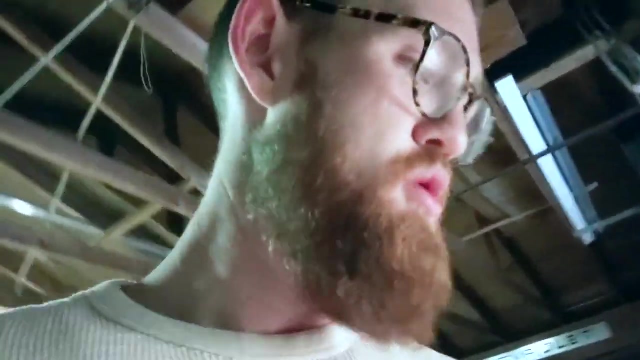 Saturday. So I had the wonderful luxury of having never frozen meat, Which is pretty cool if you think about it. What is this? Bones? Make some bone broth with that, With our own lamb. How cool is that? More bones, Okay. 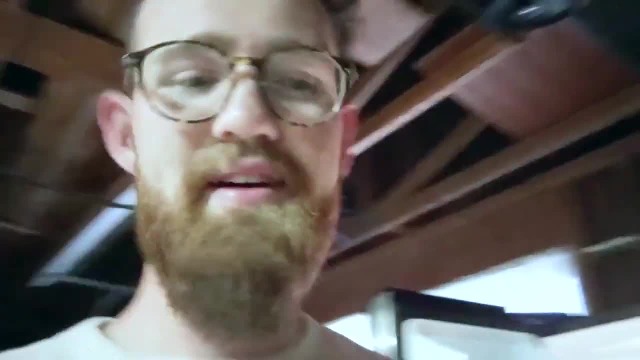 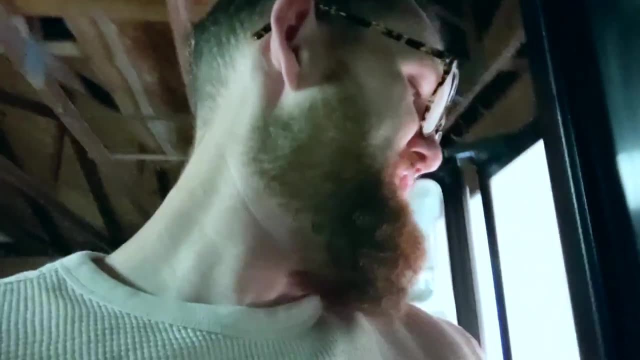 this next box is kind of like all the ofal and stuff. Here are the testicles. I don't know why we kept those. It just felt right to do. We have a few options for plans of things to do with the testicles. 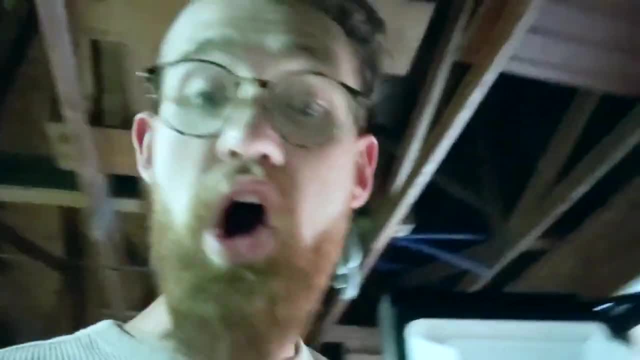 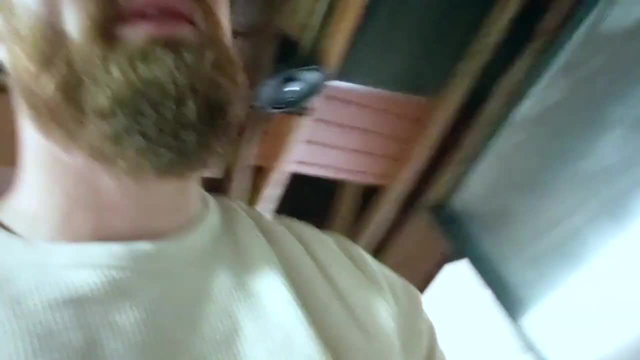 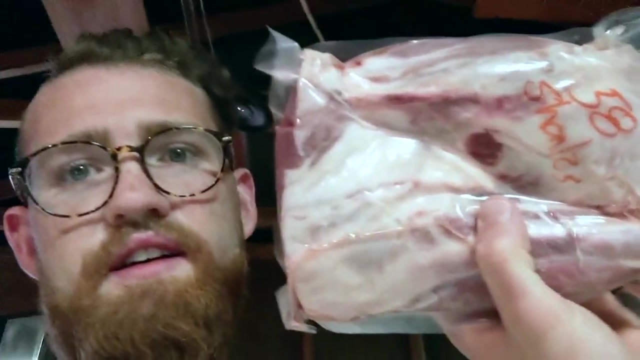 Look at that liver. What the heck is this? More bones. I actually didn't know I had that much. I guess there's two packages of bones per lamb, Because these look like bones too. They are All right. Oh, the shanks. Look at that. That's so pretty. That first thing that I thought was a 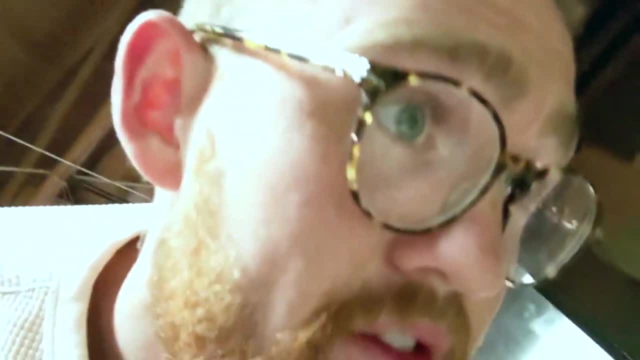 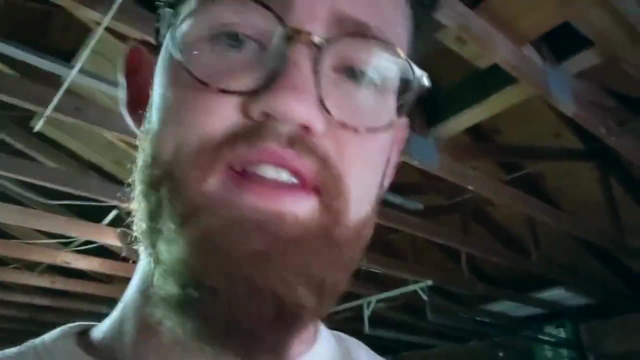 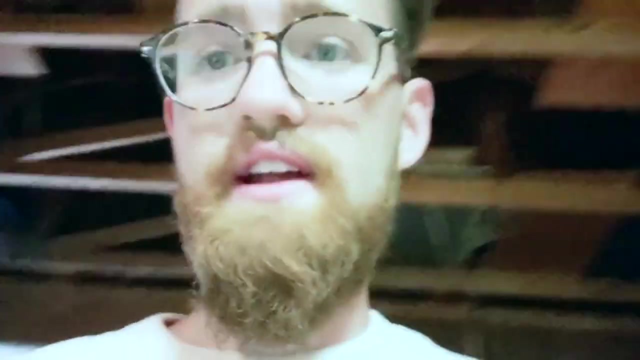 shank is a neck Bad on me for not knowing anything. Okay, so this next box down here kind of all like the little chops and stuff like that. Look at these, Maybe not right next to the fridge. Look at that, So excited for those chops. Oh yeah, Here's the other shanks, A little braised. 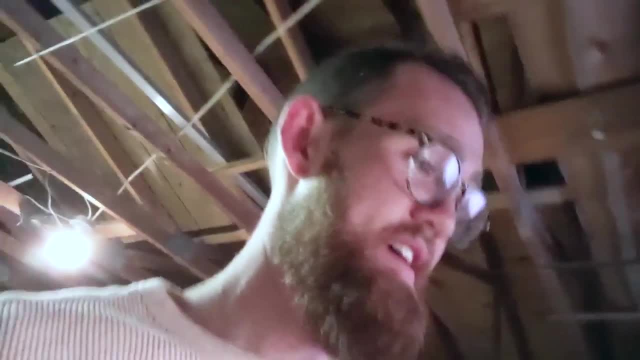 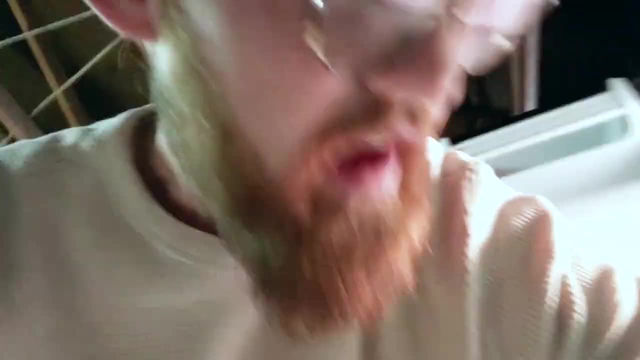 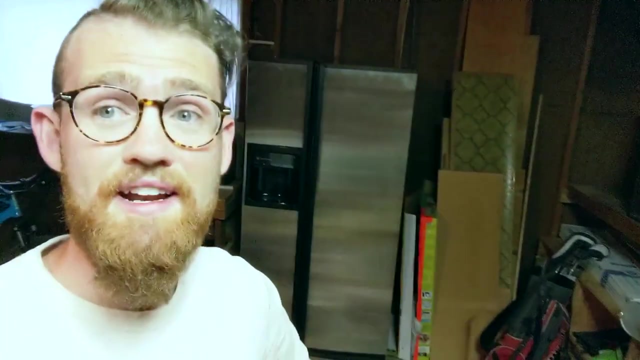 lamb shank action. That's going to be delicious. Lamb chop right there, So good. I wish I knew more about where this all comes from on the sheet. I think that will come in time. More rib chops Looks so good, Man. I really wish I cleaned my garage before this. But you don't care, You're. 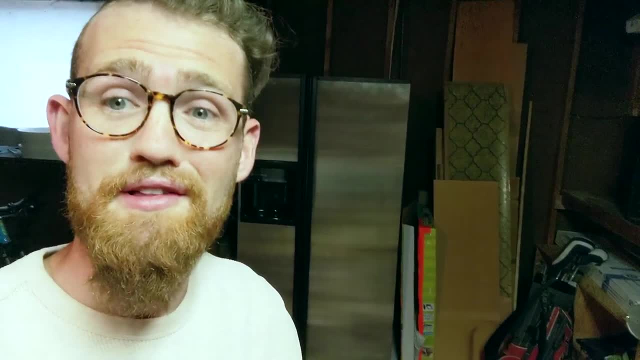 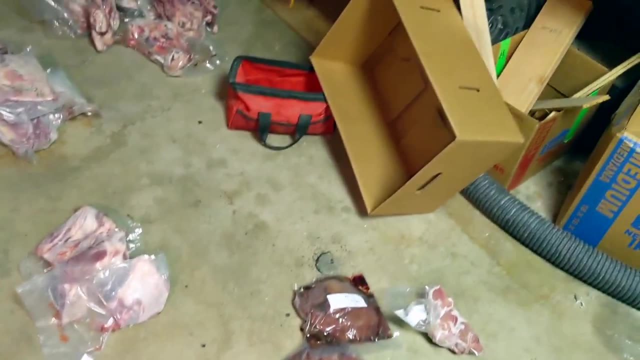 just here for the lamb. Let me show you really what this all looks like when it's all said and done. Okay, so this is what it all looks like. Pardon, the golf clubs and the empty toolbox and the empty box box just hanging around here. But let's take a little walkthrough of what we got. 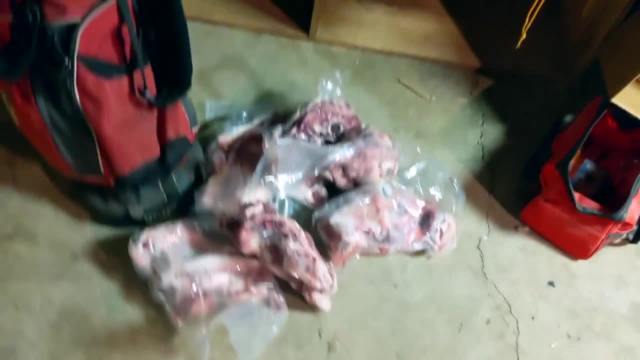 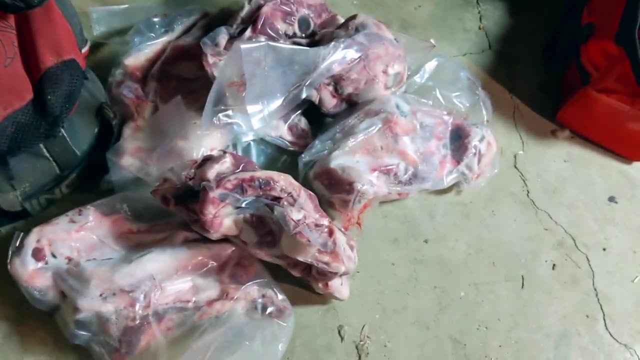 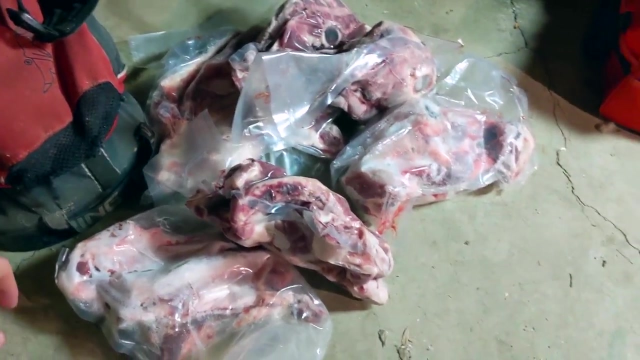 here. This pile is kind of the spare parts. This is all bones. This is all the shanks, This is all bones. So these are bones and skulls from two different animals. The guy that I gave my other lamb to does not care for this stuff, So more for us. So what that means is I've got two bags of 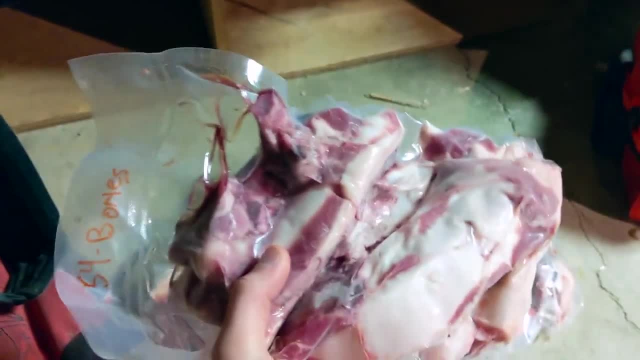 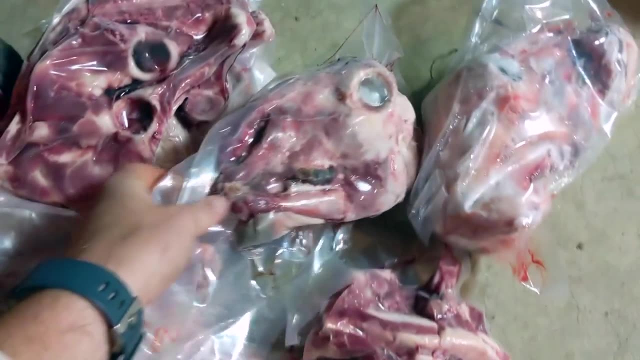 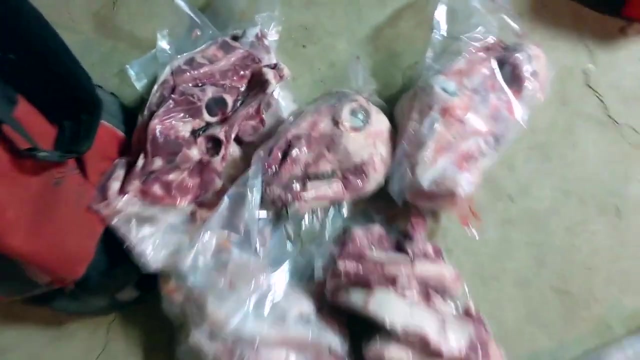 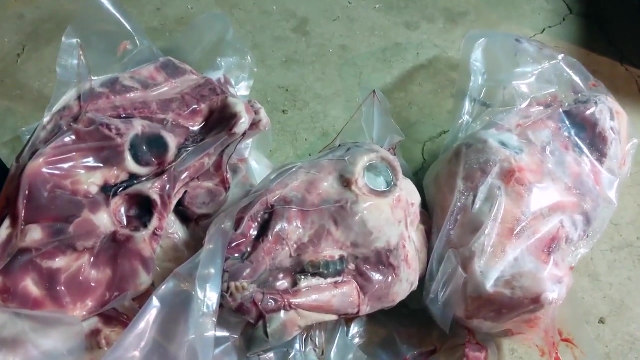 bones like this, Two bags of these for each lamb, And then that's bones, And then a skull, Which I will talk about later. No, I'll just talk about it now. Basically, the idea is, you take a skull like that and during the wintertime, when it's nice and cold outside, you feed it to your 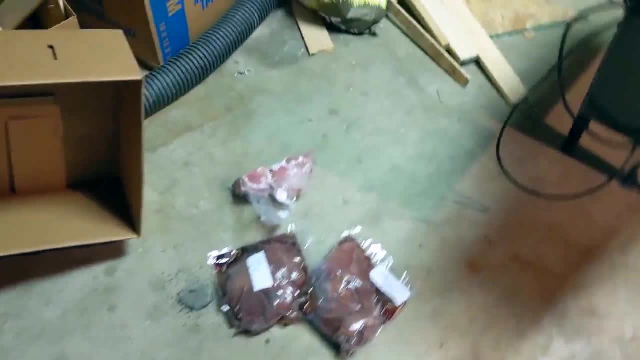 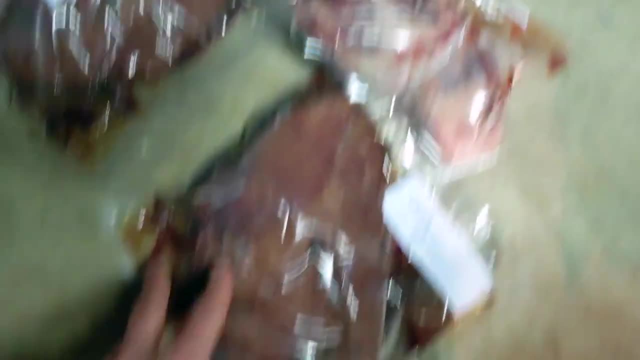 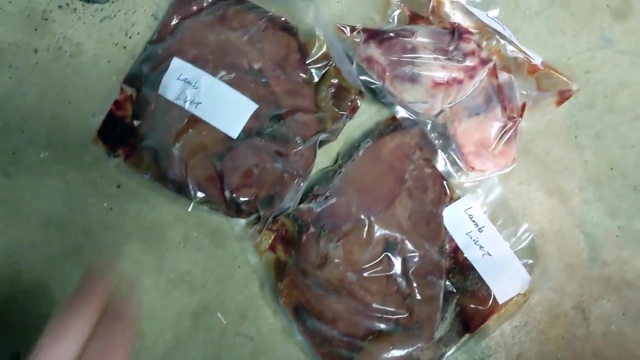 chickens and let them peck at it in the snow Sounds gross, but nothing goes to waste Here. and speaking of nothing goes to waste, I've got the livers which I accidentally took my neighbor's liver That I was supposed to give him. So obviously two sheep don't produce four livers, But we've got. 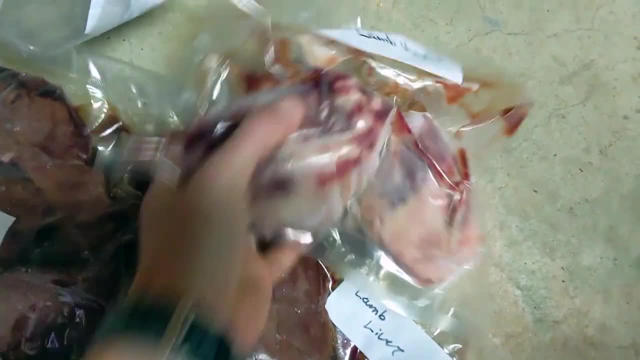 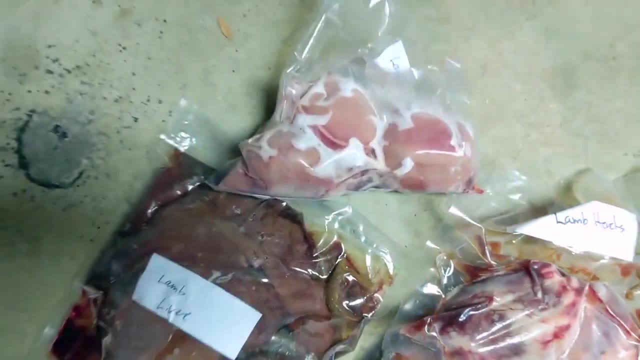 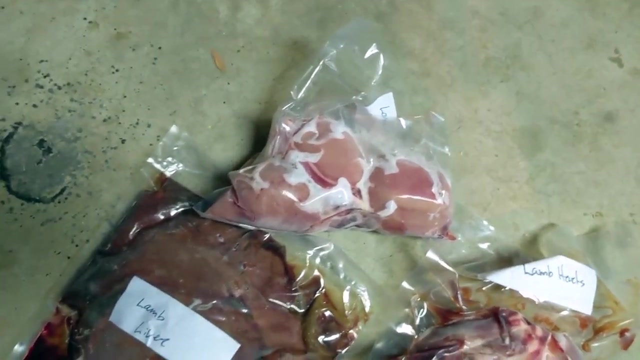 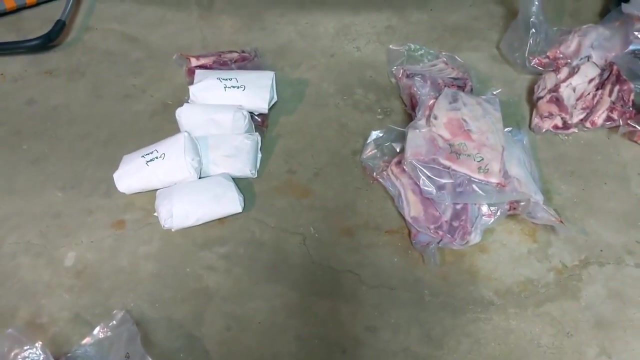 liver right here. And then these are the two hearts from these two lambs And the testicles, which there are three in there And I don't know why. My butcher said he doesn't know where the fourth one went. So I'm a little bit nervous about that ground beef over there Or, sorry, ground lamb over there. 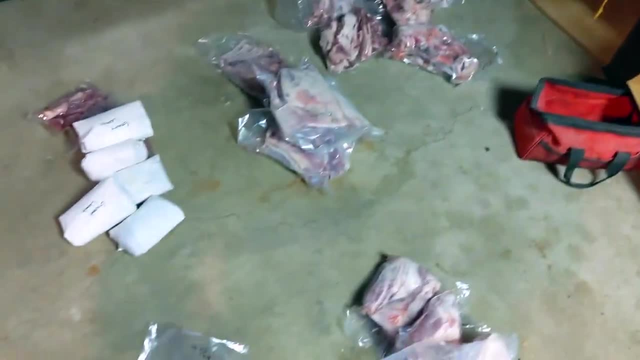 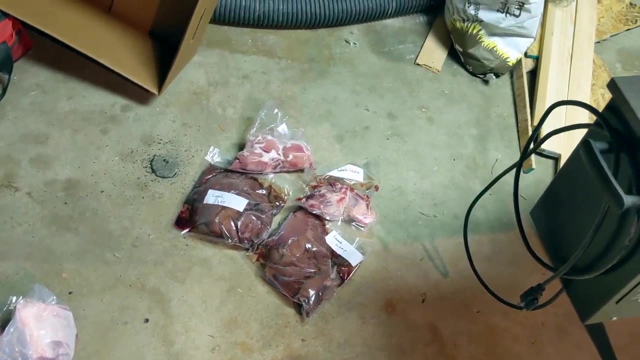 I don't know. Anyway, there's a few things we can do with that ofal, But always worst case scenario, you cook it and or basically it's chicken food if you want it to be. However, I do want to try. 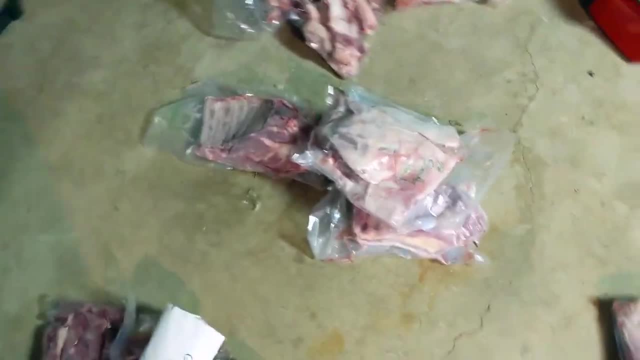 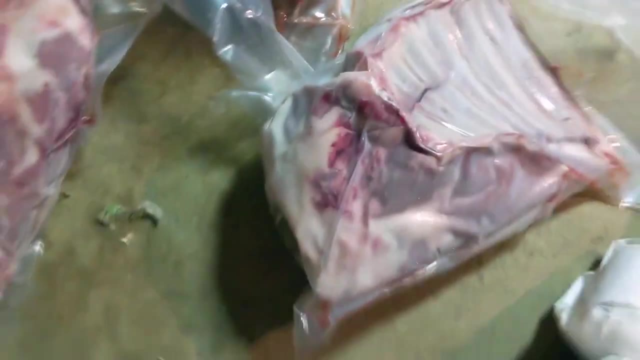 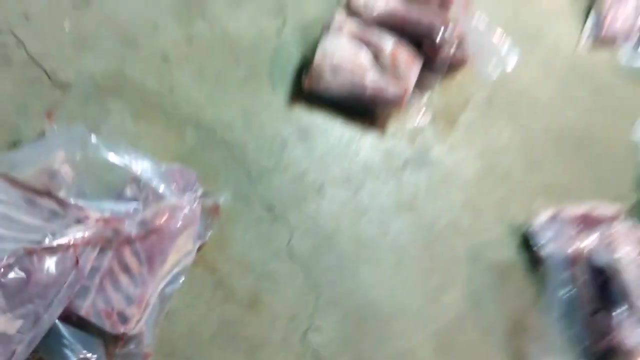 I want to learn to like liver. Okay, this pile right here Is the four shoulders. Just beautiful cuts right here. Do these nice and slow and low for a special occasion. Really excited for these cuts. The shanks and the neck over here, That's a pretty good. 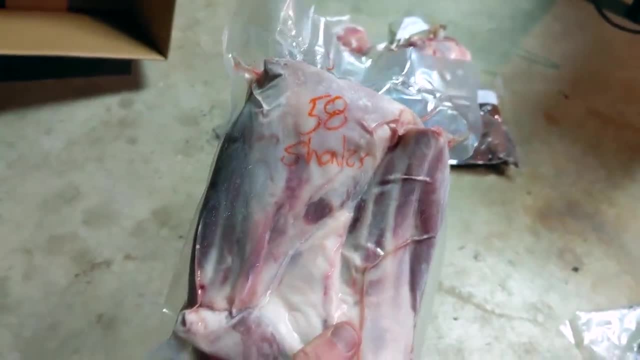 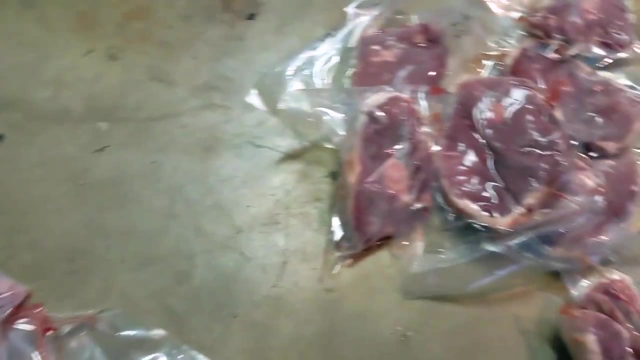 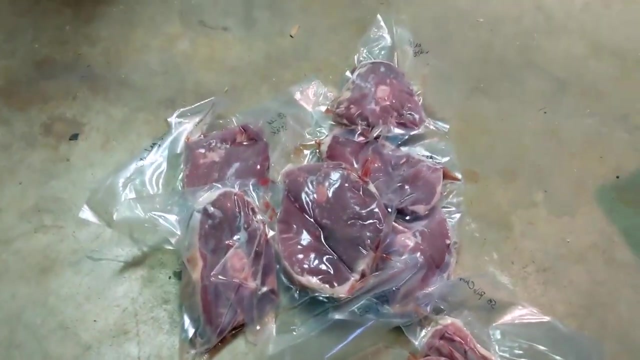 size shank man For a six-month lamb, Really happy with what these look like. That neck very similar to a shank. Oh, all the steaks. So I had two steaks. Sorry, my family had two steaks. I just ate one of them by myself. 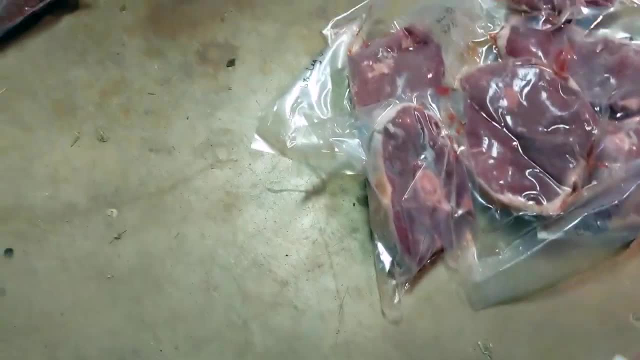 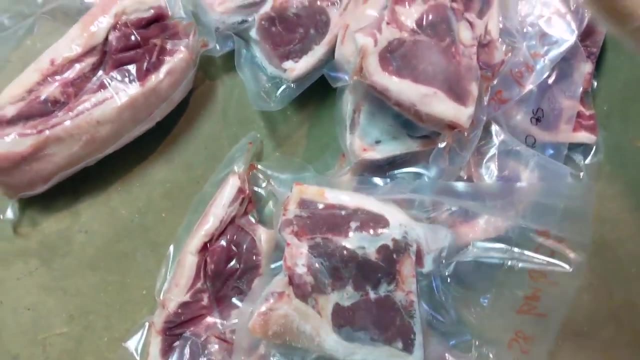 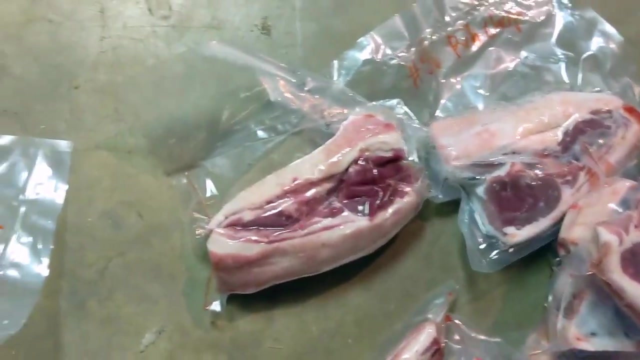 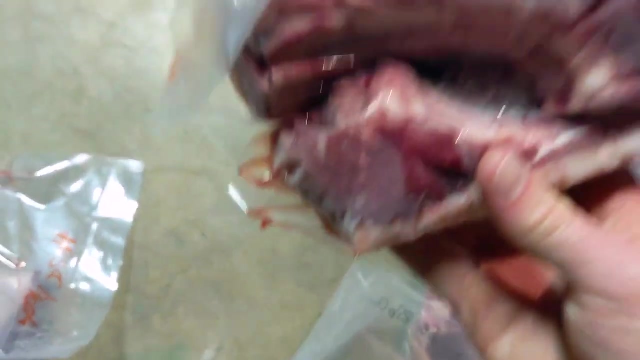 Delicious. Dorper is so good, Oh my gosh. And then there's the ribs and all the chops over here. So what is this right here? Lamb chops- How good do those look? Let's see what we got here. Yeah, these guys right here. More rib chops- So good, I think that's the equivalent to a tomahawk. 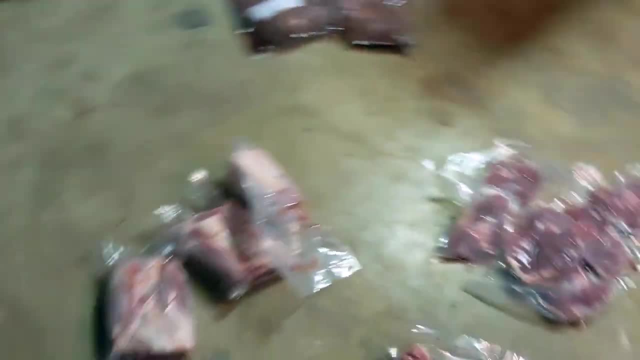 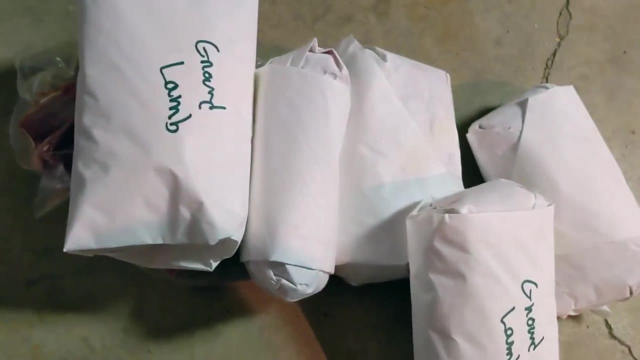 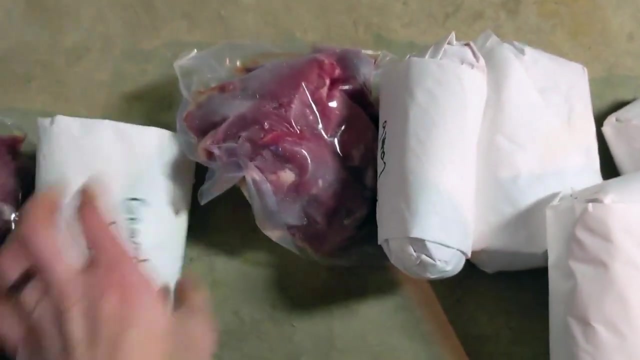 steak for a cow And then back to just the ground lamb and the stew meat. Not that much, Isn't that surprising. I had no idea that I would only be getting five pounds basically of ground lamb. And what's that? Two pounds, Yeah, those weigh the same Two pounds of stew meat. 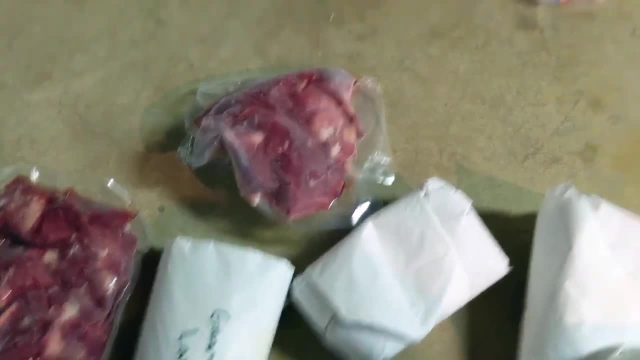 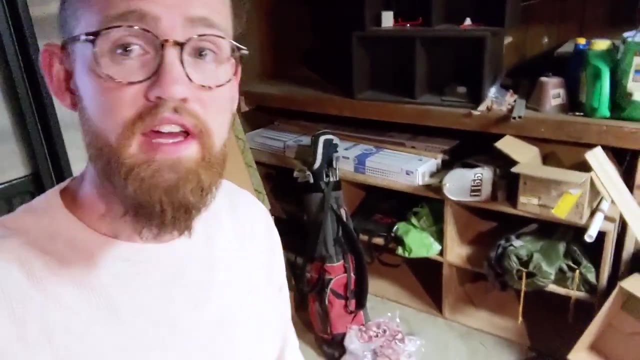 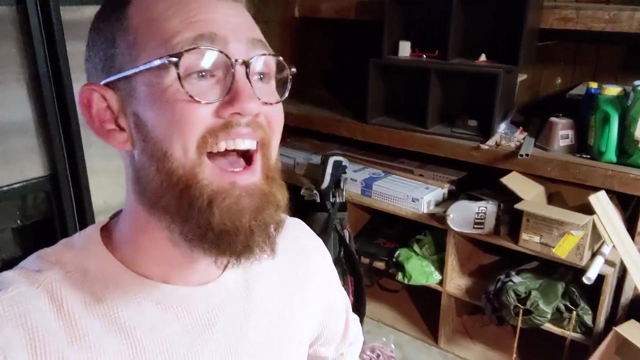 Crazy, right, Okay. so when all is said and done- and I have not weighed these all myself- it looks like I'm looking at about 50 pounds of meat. Maybe I'll just play it safe Between 40 and 50 pounds of meat. I did not get a live weight. 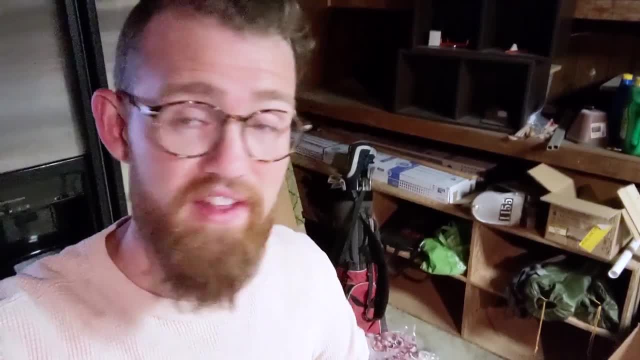 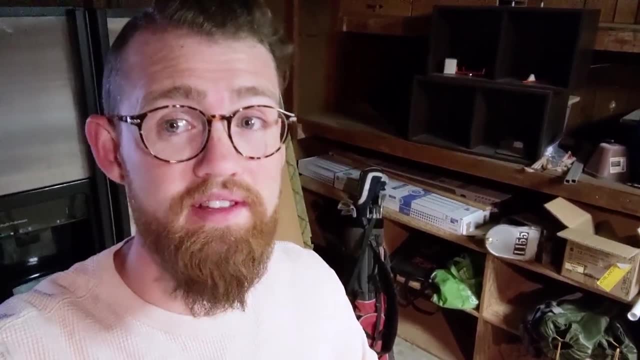 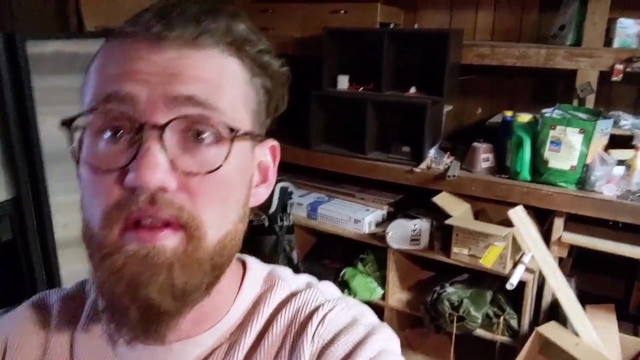 on my lambs before they went out the door. But if their hanging weight was 54 and 58, I'd imagine they were close to 100 pounds, Which is great, This butcher that I found it was so cool to be paid this compliment. 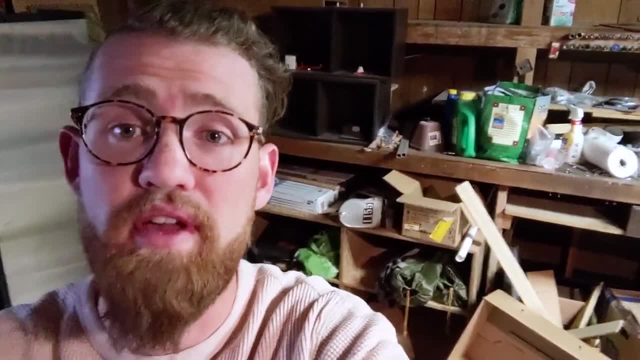 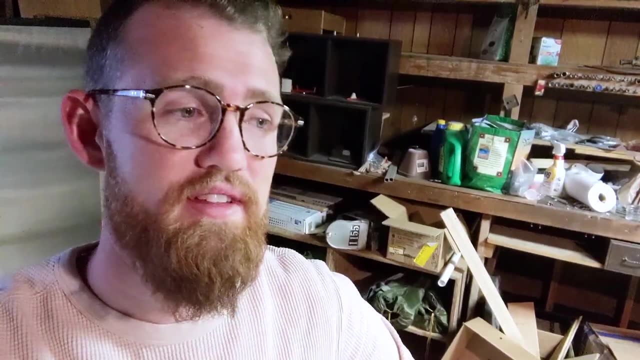 but he said: you know, whatever you're doing with these sheep, keep doing it. And that really meant a lot to me. He just said that their marbling was better than what he typically sees Very lean. I think a lot of that. the leanness has to go with their age, But again, it just proved that. 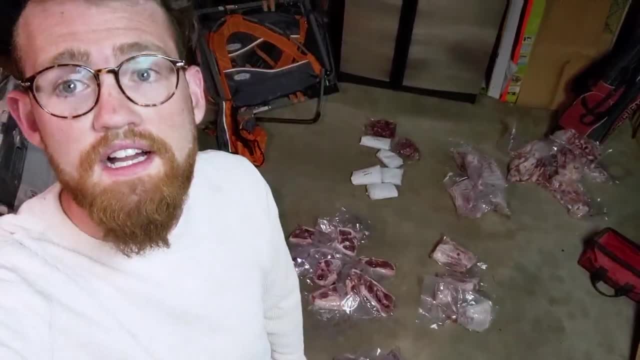 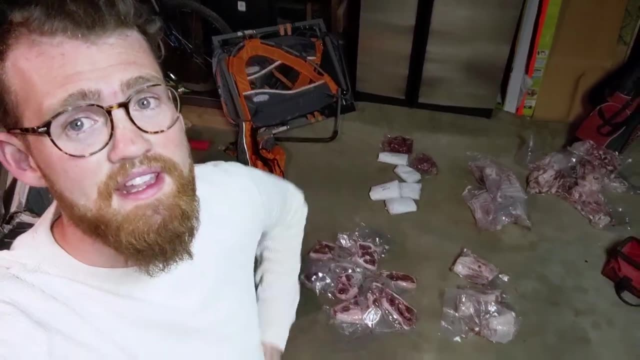 it's viable to do it with a six-month lamb. Very, very cool. Another plug to say: don't look at my messy garage, But if you're interested in lamb, I recommend it. If you were like me a year ago and you didn't know how much you were going to get.